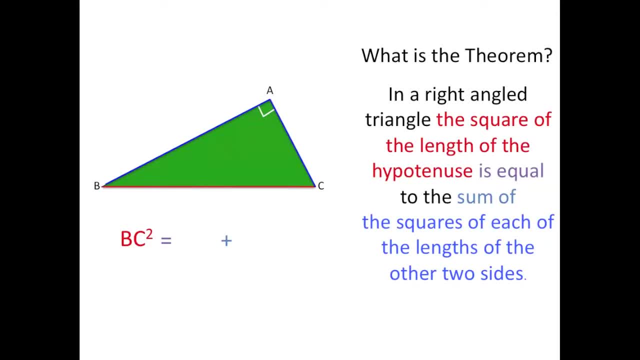 AB and AC, And again we're squaring each of these sides. So we're going to end up with AB squared and AC squared, And thus the theorem basically means that BC squared is equal to AB squared plus AC squared, And this is what we want to prove today. 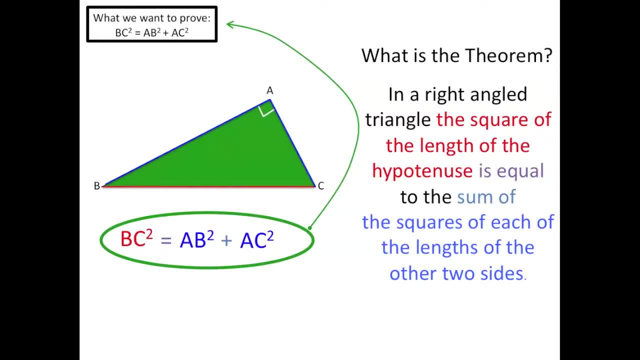 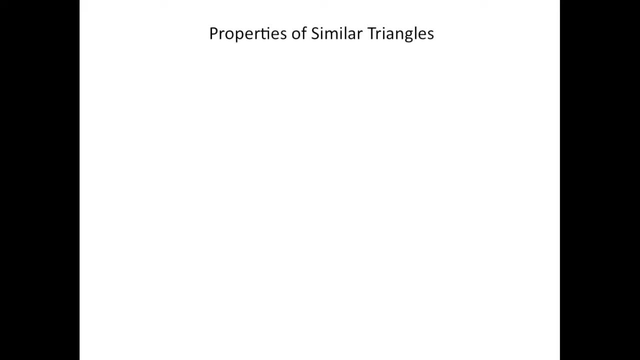 So we'll write it up here for reference. So, before we get into that, to understand the proof that we're about to do, you need to understand the properties of similar triangles, Because the proof we want to use uses similar triangle properties. The first. so we have our two similar triangles, X and Y. 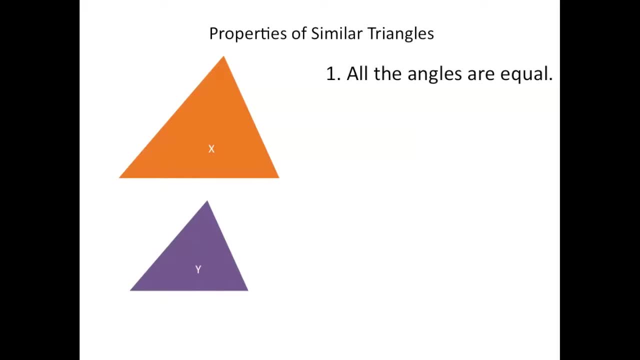 The first property of similar triangles is that all the angles are equal, So let's label each of the angles. We have PQR, And then, for triangle Y, we have TUV. Now, though, I have told you that both these triangles are similar. 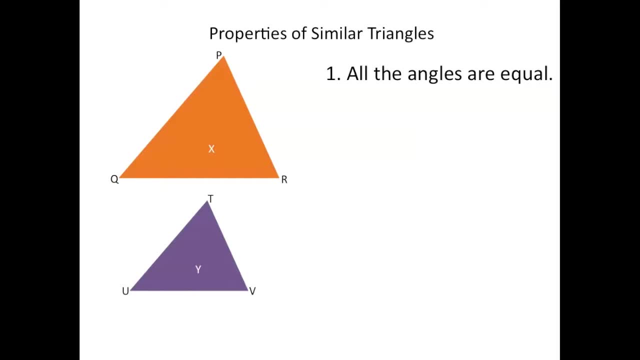 let's place triangle Y on top of triangle X to confirm whether their angles actually are equal. So first let's see if P and T are equal And, as you can see, angle P and angle T fall on top of each other perfectly. 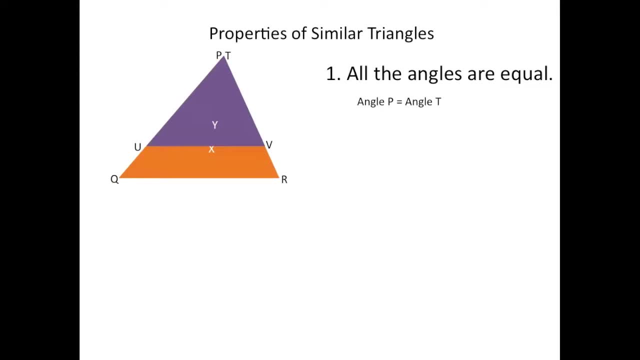 So that means they're equal. Next, let's try Q and U. Again, they fall on top of each other, perfectly meaning that they're equal. And lastly, we're left with angle V and angle R, And of course they fell on top of each other. 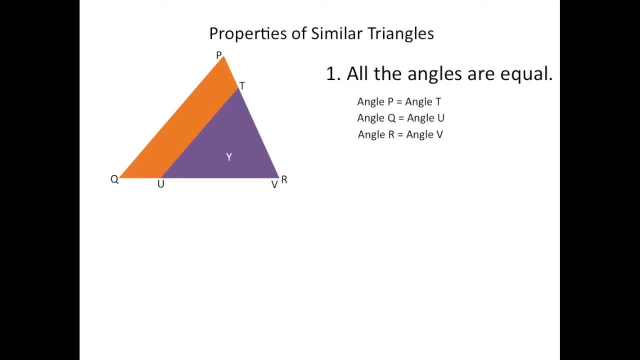 showing that all three angles in both these triangles are equal. So we can write out that triangle PQR is similar to triangle TUV. One interesting thing about triangles is that all their angles add up to 180.. So in triangle X, P plus Q plus R gives you 180 degrees. 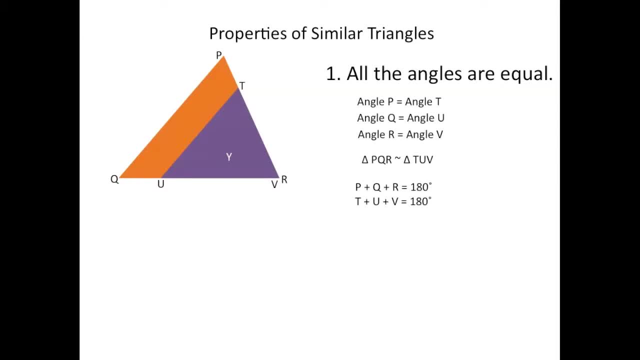 And in triangle Y, T plus U plus V gives you 180 degrees. So if you notice the moment when we showed that P is equal to T and Q is equal to U, then automatically R must be equal to V, And this is knowing. this is very convenient because 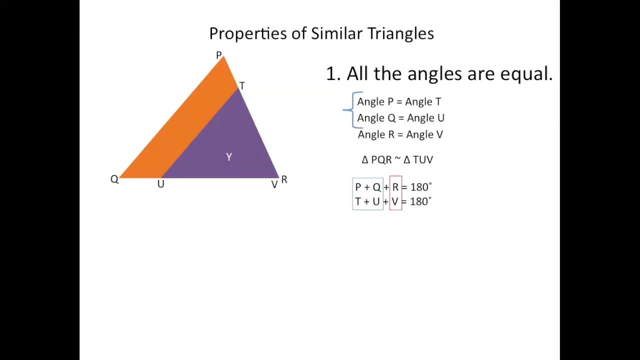 then in the beginning, when we showed that angle P was equal to angle T and angle Q was equal to angle R and angle Q was equal to angle U, we can automatically jump to this step and say that the two triangles are equal. 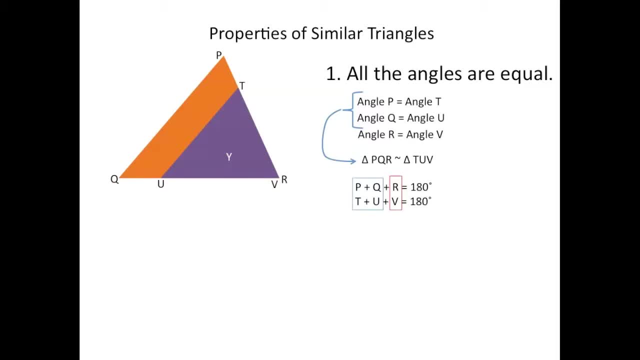 instead of going to the third step and saying that angle R is equal to angle V, because it is assumed that they must be equal since the first two angles were equal, And this is known as angle-angle criterion for similar triangles, and it's usually written shorthand as AA. 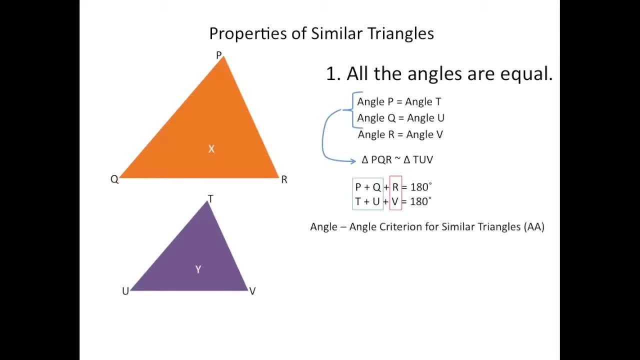 Now the second property that we're going to need is all the sides of the similar triangles are proportional, which means that the corresponding sides can be written as ratios to one another that equal each other. So, for example, we're going to start with the big triangle. 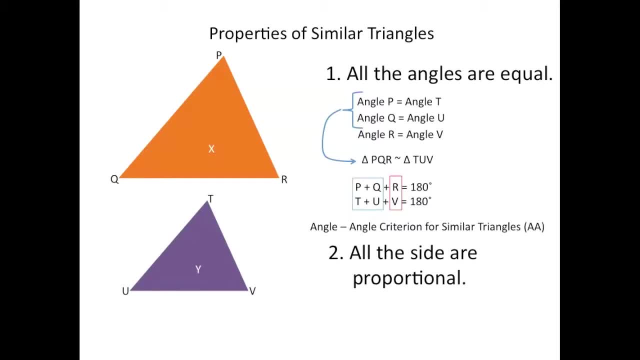 and write the ratios of the length of triangle X versus triangle Y And we'll get: PQ over TU is equal to QR over UV, which is equal to PR over TV. Again, both these concepts we're going to need later on when we start our proof. 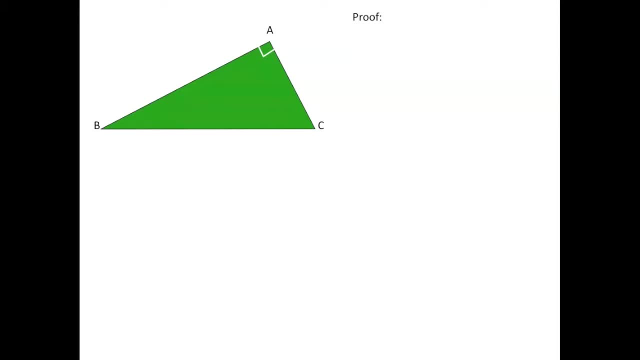 So now back to our proof. And what were we trying to prove? That BC squared is equal to AB squared plus AC squared. So the first thing I'm going to do is draw a straight line, a perpendicular line, that is. 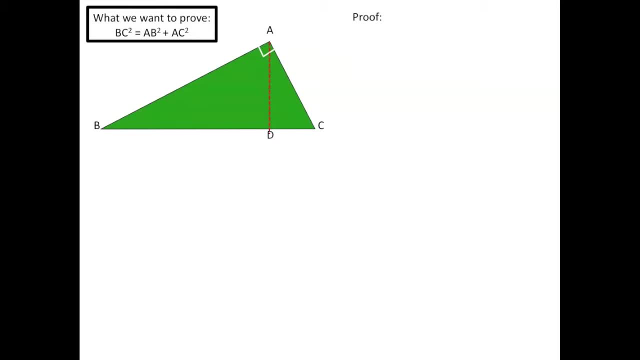 from A and label that point D. Now, if you notice, when I did this, I ended up with two smaller triangles, And both of these are also right-angled triangles because D is a perpendicular line. So let's first focus on triangle 1 at the moment. 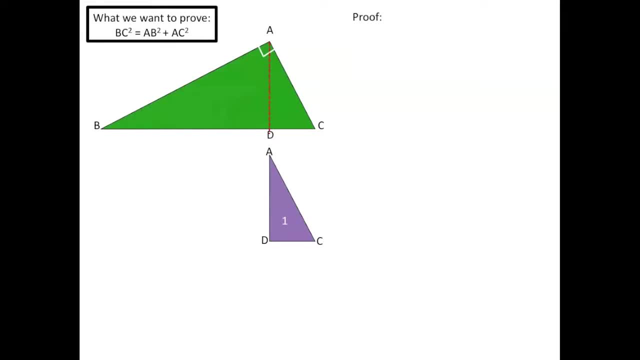 and label it accordingly, And forget about triangle 2 for now. Now we want to show that ADC is similar to ABC, And this may not be apparent at first, but let's flip and rotate this triangle to see which angles are similar and which are not. 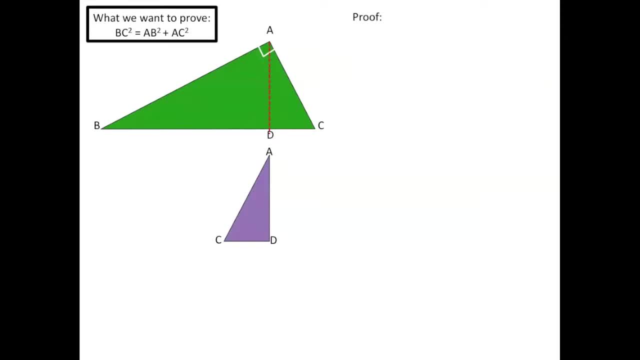 So if I flip it, notice that the labels flip, And now I'm going to rotate it. Now the triangles look much more similar, But just saying that they look similar doesn't prove that they're similar. So first thing we need to do is: 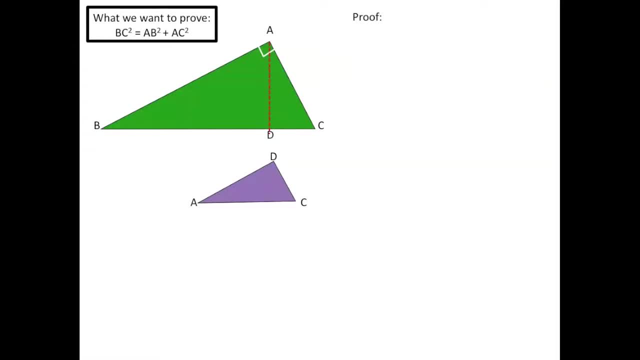 since we said earlier that because AD is a perpendicular line, that means angle D must be 90 degrees, And we also know that angle BAC in the green triangle is 90 degrees. So those two triangles are equal, meaning that they're similar. 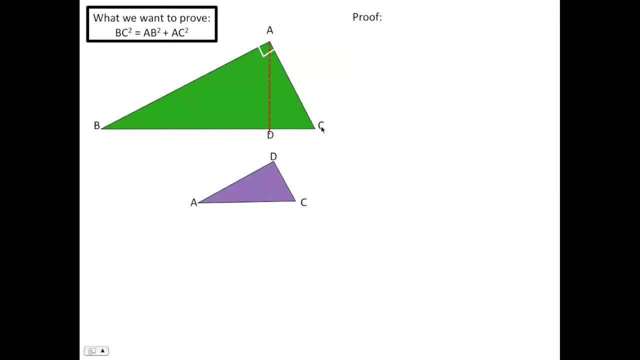 And since angle C in the green triangle here is the same angle C here, then obviously they are equal. So again by angle-angle criterion, we have that triangle ABC and triangle DAC are similar And we can write our formulae as shown. 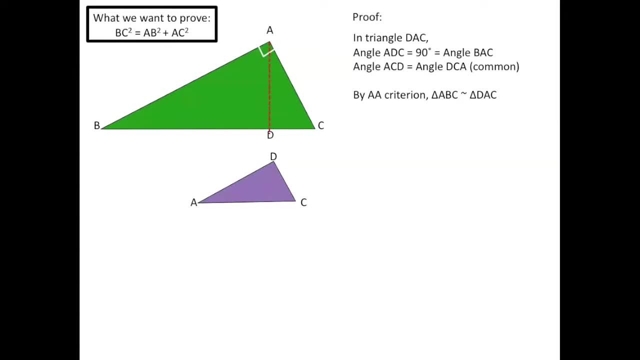 Next thing we want to do is we want to write out the proportions that we got of the two triangles, because they're similar. So I'm going to start off with the sides of the green triangle versus the purple triangle. You can do this the other way around. 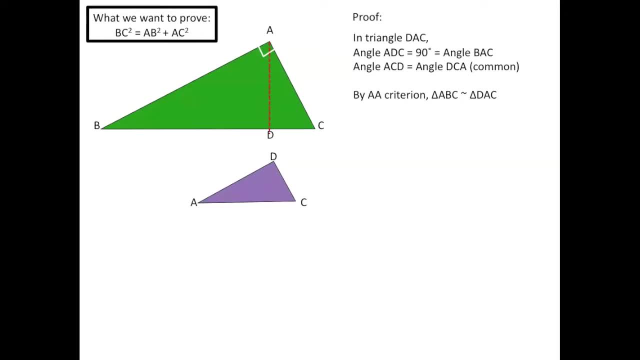 and still end up with the same result. but it's important to stay consistent. So first we're going to have: AB over DA is equal to AC over DC, Which is equal to BC over AC. So we could just leave the proportion as is. 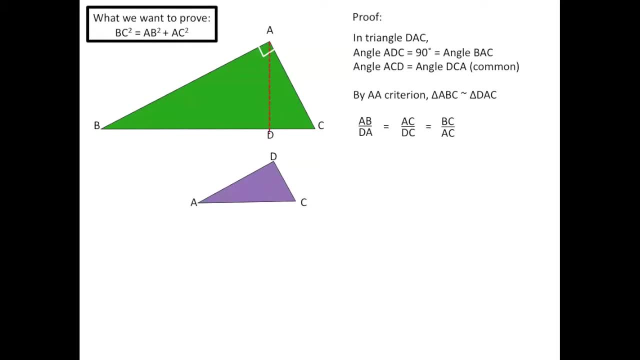 but we need to notice that we may not need all of this proportion, And to know which part of it we don't need is by looking for which part of the proportion has the line AD in it. If you remember, we're trying to find a relationship. 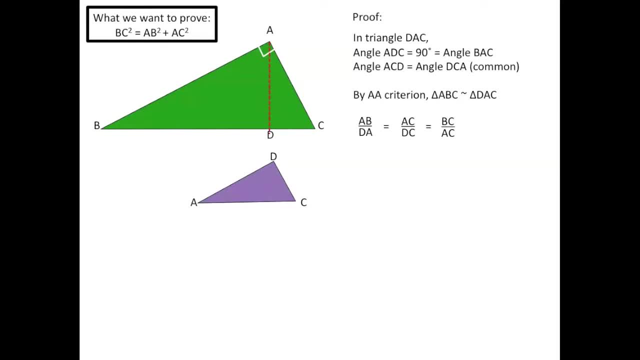 between the sides of the right angle triangle, And so side AD was created by ourselves, And it's not really associated with the triangle we had originally. Thus, anything that has AD or DA we can get rid of, And then that leaves us with the rest of the proportion. 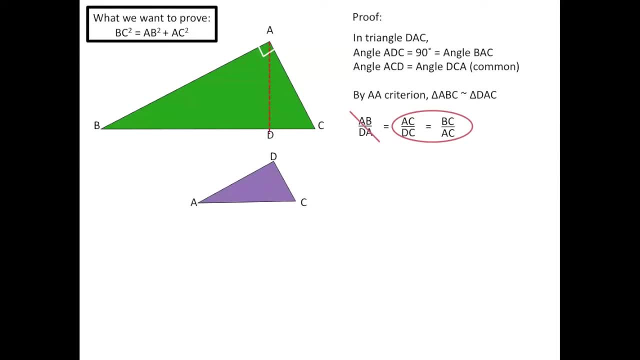 With this part of the proportion, you can now do the next step of the proof, which is cross multiply. So when you cross multiply, you end up with: AC squared is equal to BC times, DC. Okay, so that's everything we can get. 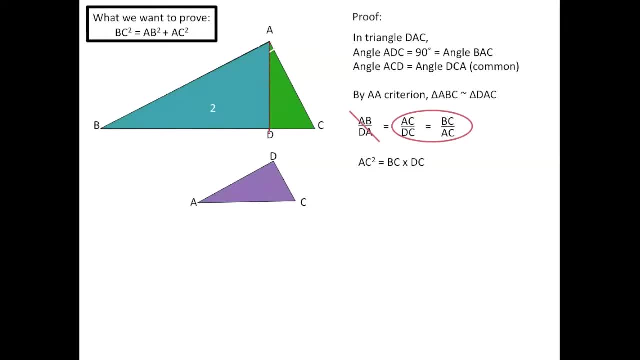 from the purple triangle. Now let's bring back triangle 2.. So again, we're going to do the same thing with triangle 2. First we're going to label it, then flip it and rotate it, So its orientation is similar to. 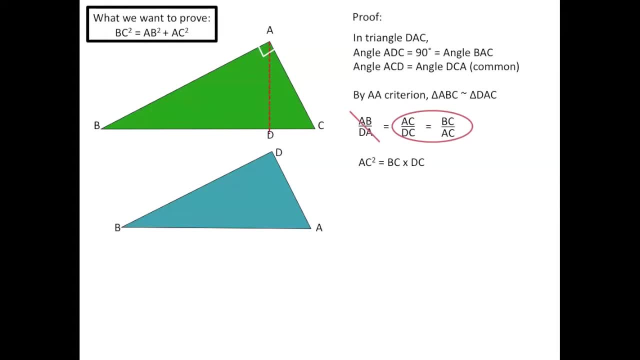 triangle, ABC. Now again we want to prove that ABC is similar to DBA. So angle D is again 90 degrees, just like angle A of the green triangle, And in this time we have this angle B. 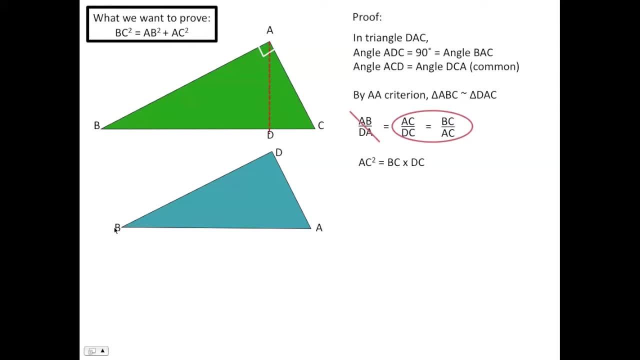 which is the exact same angle B over here. So since these two angles are common and these two angles are 90 degrees by the angle-angle criterion, we know that triangle ABC is similar to DBA. Again, we can write it out formally: 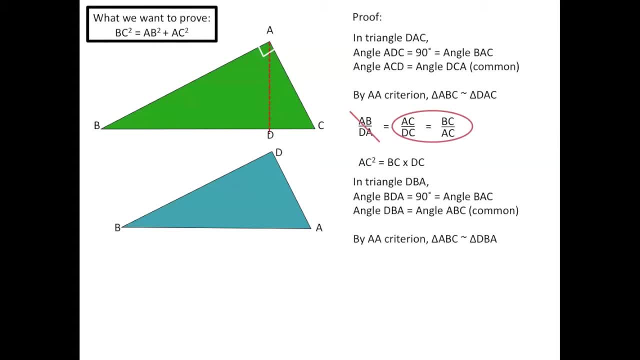 as shown, And this time we're going to write out our proportions the same way as we did before, So we'll end up with: AB over DB is equal to AC over DA is equal to BC over BA. Again, we're going to cross out. 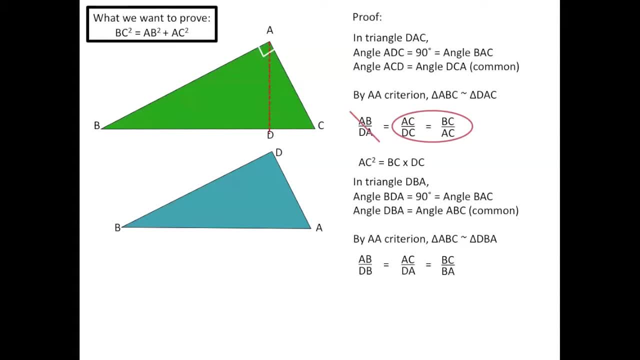 the part of the proportion that has a DA or AD in it, since that's the line that we actually added ourselves, And that leaves us with these two parts of the proportion And we'll cross-multiply. Notice that when we cross-multiply. 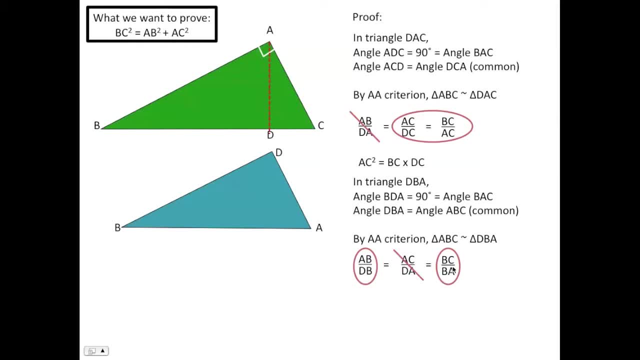 we have an AB here and a BA here. These are actually the exact same thing. it's just a different way to represent the same line. So when we cross-multiply, we're going to end up with AB. squared is equal to DB times BC. 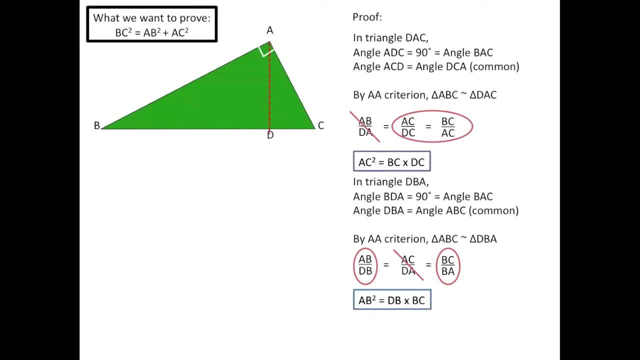 Now we finally have the two equations we need to do our proof, So let's write them out over here, And at this point you may get stuck in what we should do first. Well, let's look back at what we were trying to prove.